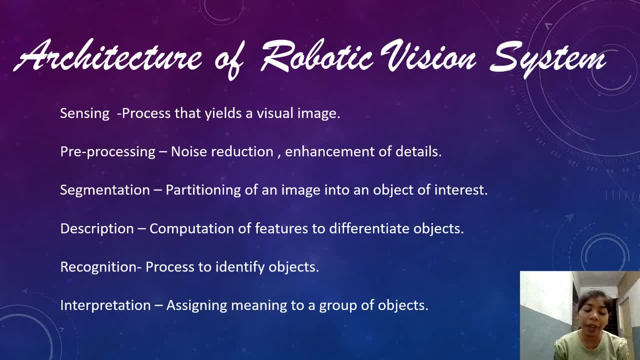 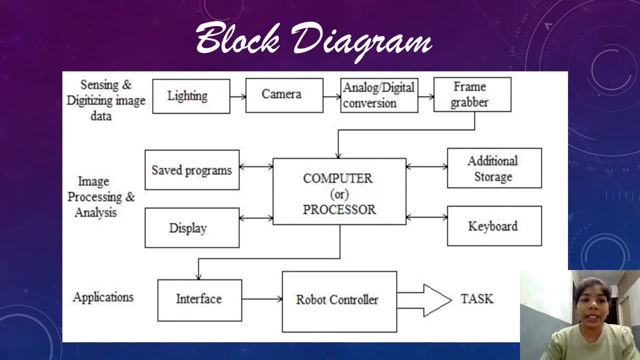 Next is recognition. Recognition is the process to identify the objects. And last is interpretation. It is to assigning meaning to a group of objects. So there is a block diagram of robot vision in front of you. This first row is of sensing and digitizing image data. 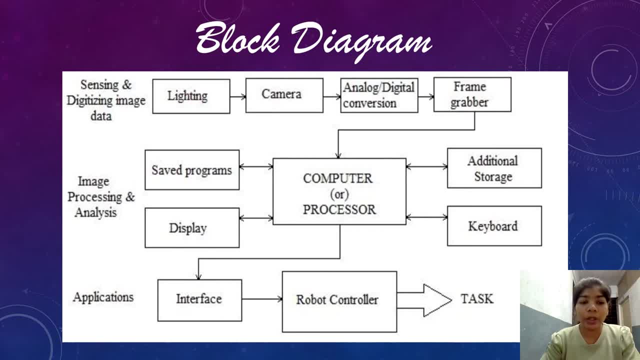 Second row is of image processing and analyze, And third one is of applications. So first light is processed into the camera and it converts the analog signals into the digital signals, And then it grabs into the frame And that all data is transferred to the processor. 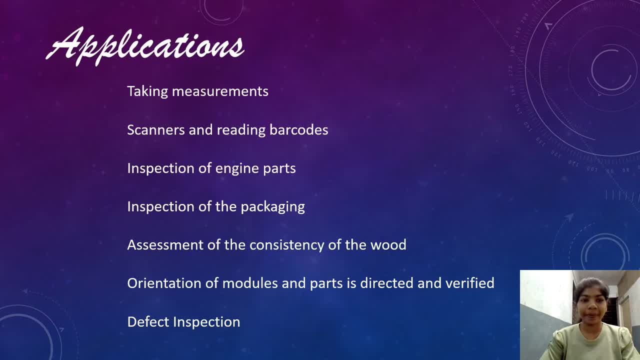 And then task is performed. So here is applications of robot vision in front of you. There are many applications of the robot vision which are in front of you. There are taking measurements, scanners and reading barcodes. infections of engine parts, infection of the packaging, assessment and consistency of the wood. orientation of modules and parts is directed and verified and defect infections. 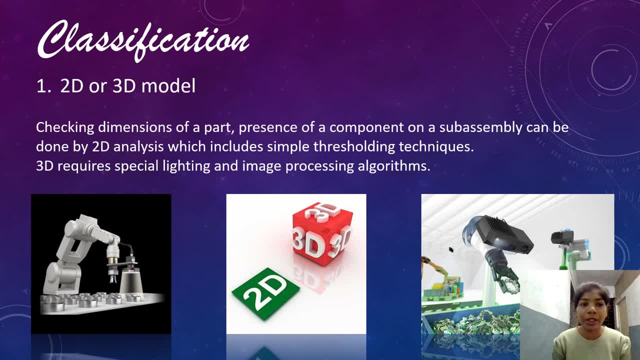 Today we are going to do classification of robot visions. First one is 2D vision, Second one is 3D or 3D models And second one is number of grayscales. So in 2D or 3D models we can check the dimension of path. presence of component on the sub-assembly can be done by 2D analysis, which includes simple ratio techniques. 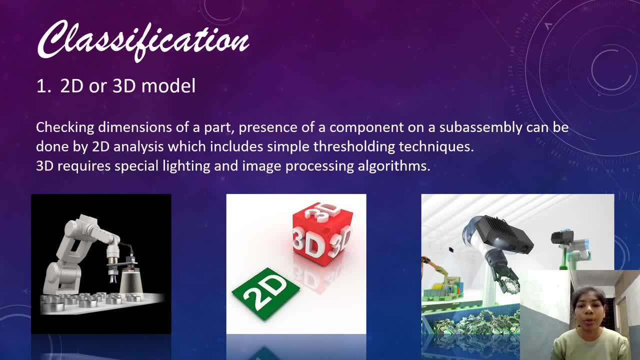 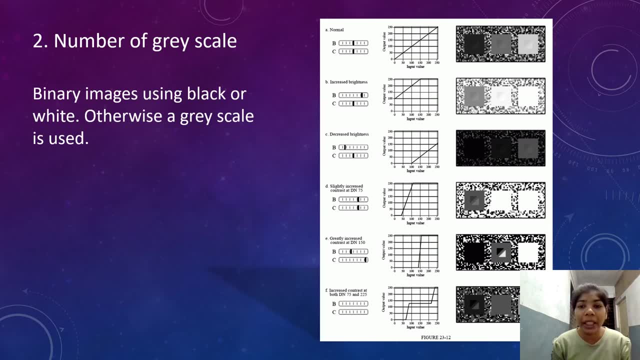 And in 3D requires spatial lightning and image process algorithms. And second one is number of grayscale. In grayscale, binary images use black or white, else whether it can also use white And in 3D it can also use gray scale. 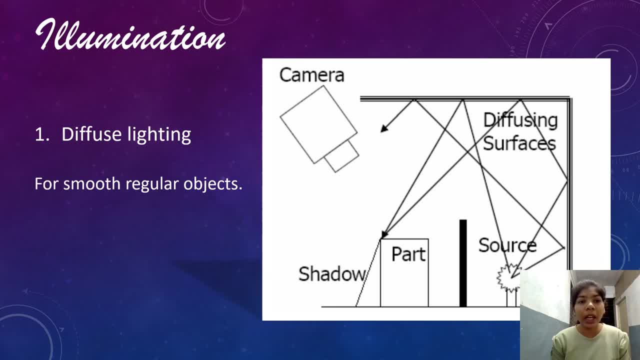 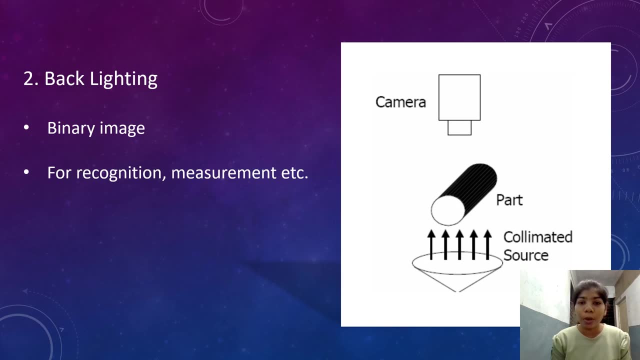 Now we are going to look. illumination of the robot vision. There are two types of illumination. First one is diffuse lighting and second one is back lightning. In diffuse lightning, which is used only for smooth objects, And second one is back lightning, which is used for binary images and for recognition and measurement and many more. 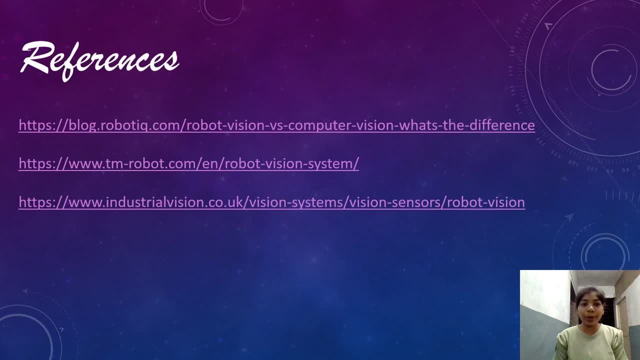 And here are the references which I have used to make this presentation. Thank you so much, guys.